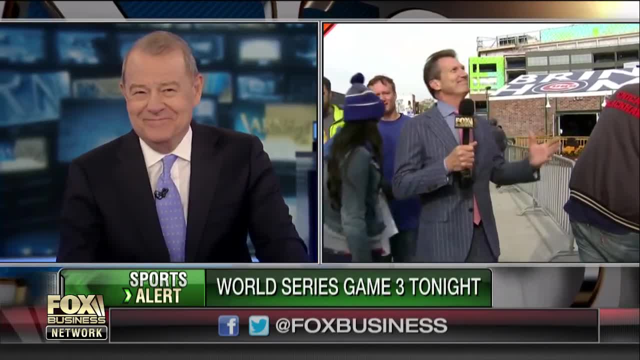 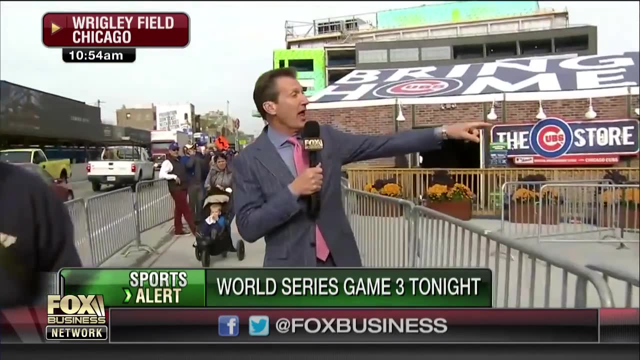 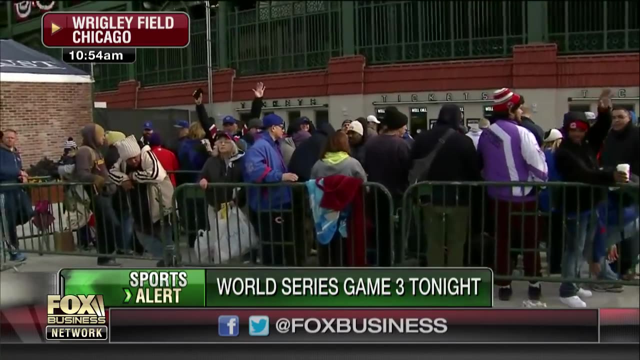 standing on hallowed ground. What are you up to? I tell you, people don't even know that the president is trying to get Cubs tickets. Look at these people. This is a line of people that think those are the will call ticket line that there may be some extra tickets.